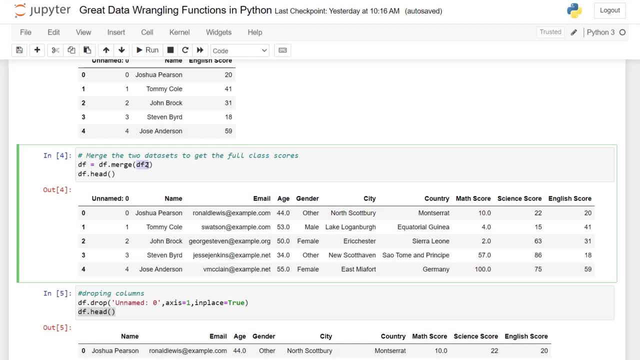 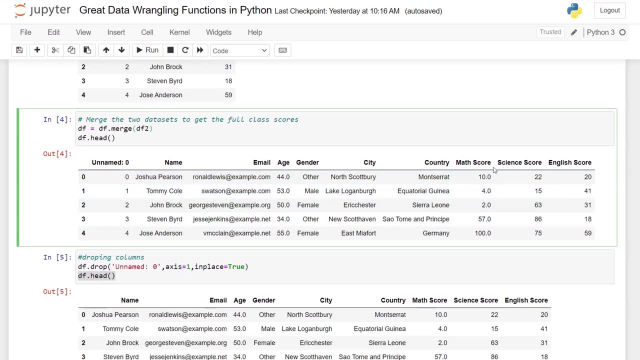 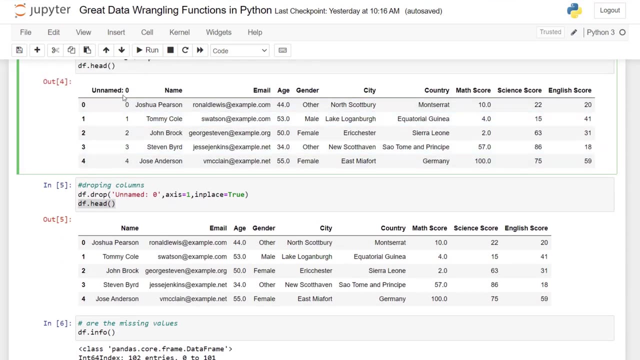 We can indicate the type of merge we want by using other parameters, but the default is inner, as you see there, And what we get is the new data set here with the English scores attached. Let's see. Let's drop this unnamed column here that we have here. 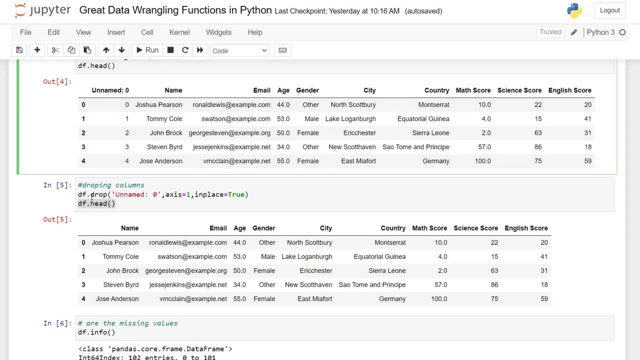 We don't need that column, so we can use the same data frame and drop the unnamed column And we want to drop the column which is axis one and we want to make sure that's done in place. And you can see, if I use the data set head, which gives us the first five rows, we can see that we were able to get rid of that column and get the new data set. 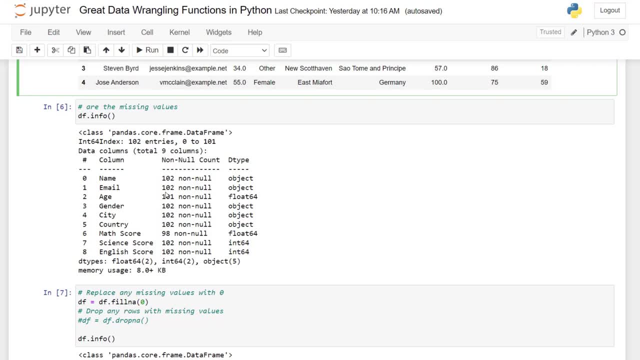 Next, we want to use info to see what null or missing values we can have. You can see we have 102 entries, but not all of the columns have full values. You can see for age we have 101 instead of 102, and 98 for our math scores. 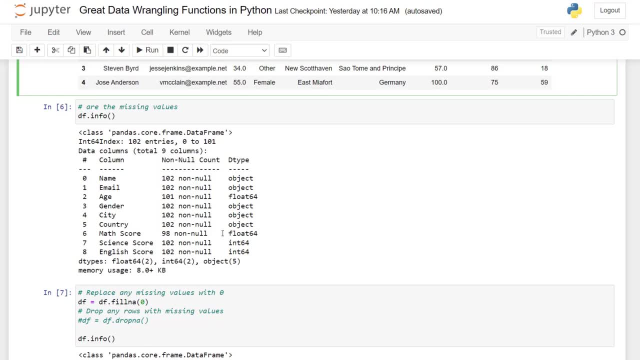 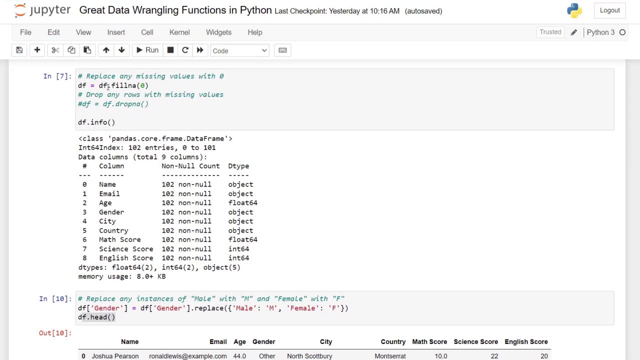 So those are both numerical columns if I look at the data types here. So I'm just going to use the fill, Same as our data set, I'm going to use the data frame function there by using fill in A and I'm going to fill any missing value with zero. 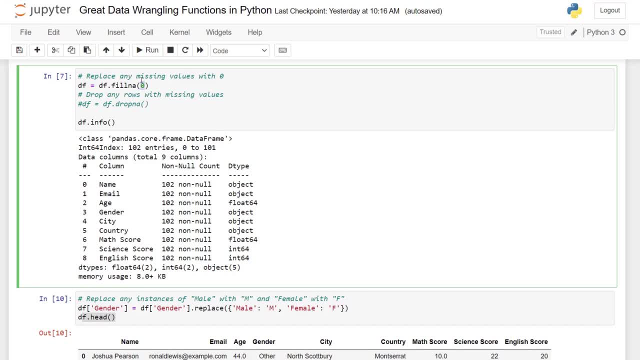 If you want, you could also drop those values. It depends on your use case. And let's look at info again to see what happened. Now you can see that all 102 have their values and we have no null values there. All of them are non null. 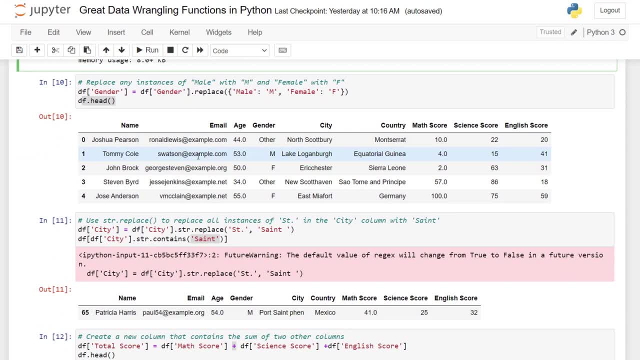 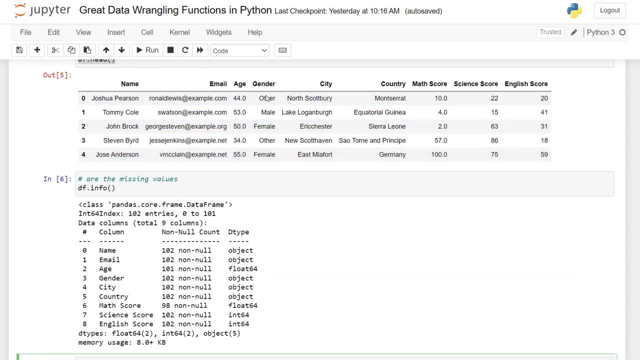 So we're going to use the fill function to see if we can get rid of any missing values in our data set. So what I want to show you next is how to replace a particular value. So within our data set, if I go back up here, we have gender and that's indicated by other male and female. 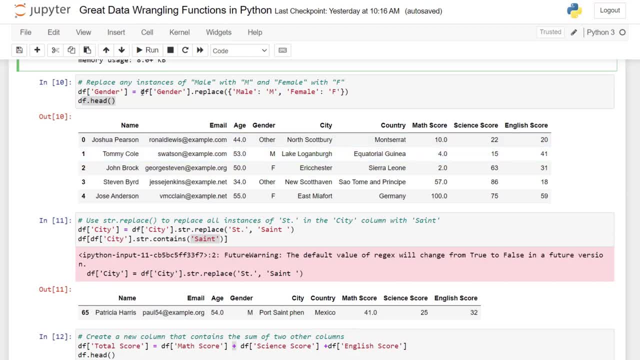 I want to replace that with just the letter M and F for male and female. I can isolate that gender column with bracket notation. Then I can use the replace function With the parentheses Where I say: anything with male, replace with M, separate by the colon. anything with female, replace with F. 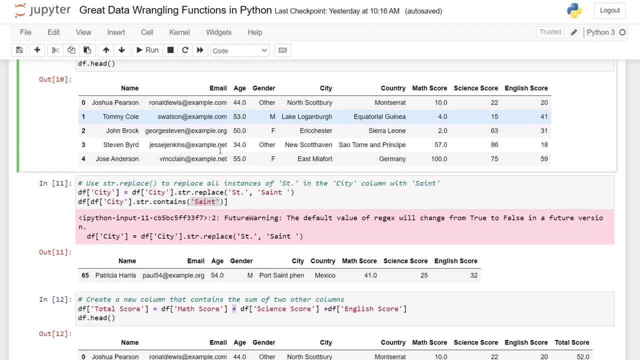 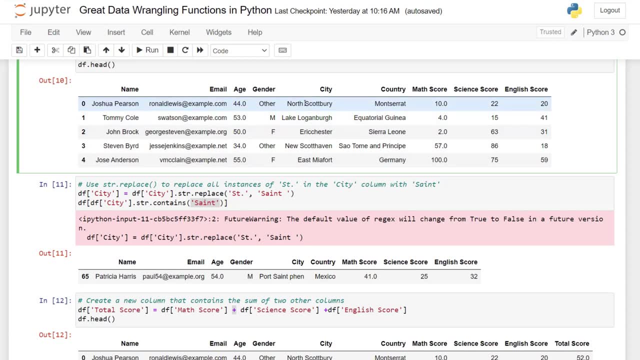 And if I look at the head, we can see that has been replaced. Next, I want to replace a specific string. So if you look here, this whole city is one text or string. I want to replace something specifically in there. I want to replace the ST. 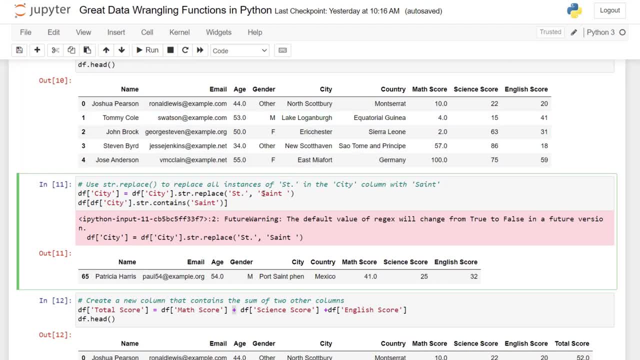 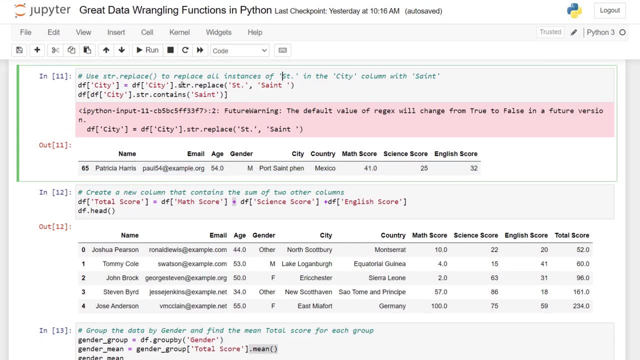 And in those strings with Saint And the way we do that is very similar. I isolate the city column, I replace it by first accessing string which is STR, dot replace, And I pass in what I want to replace, which is ST period with Saint. 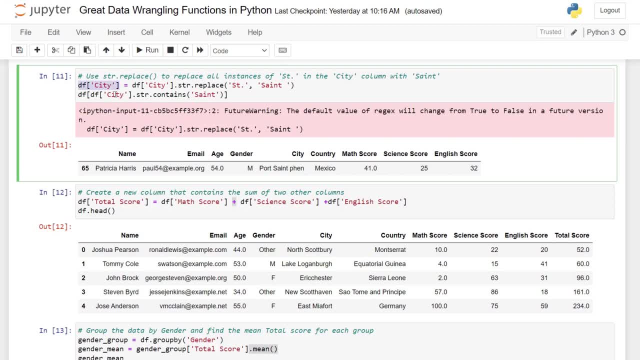 And then I reassign that city column So it just replaces everything. And then What I want to do is find that specific value. I use the string method again and look for contains anything. I renamed the Saint and you can see that has been renamed there. 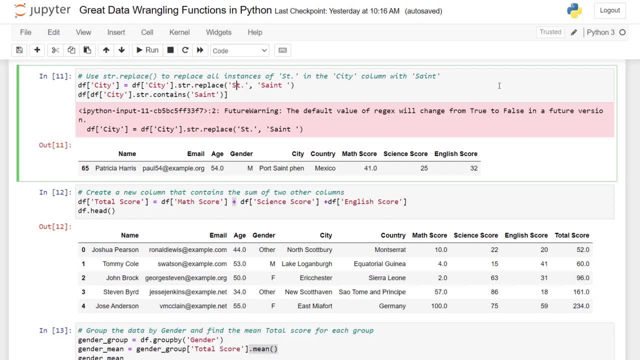 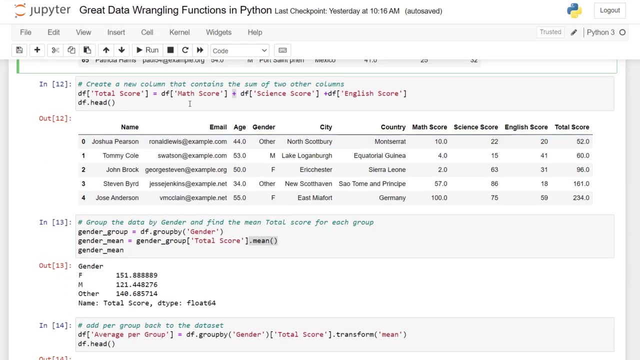 So that's a very easy way to do that. This warning is just because this is going to change in the future. Next, let's create a new column, and we can do that just by using bracket notation, passing in a new name and then doing an addition. 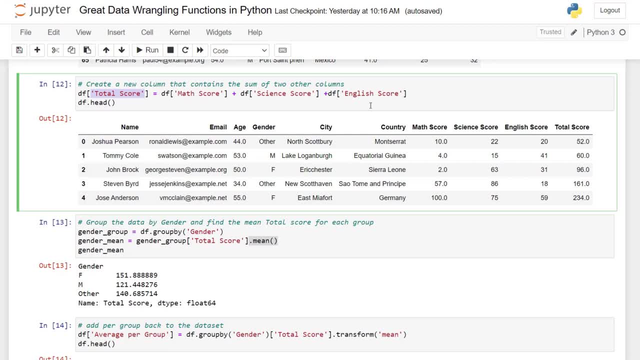 To get the total score. So I'm going to add the math, science and English score columns and then add that back to a new column that doesn't exist in the data frame, called total score. If I look at the head of our data frame you can see we now have the total score column. 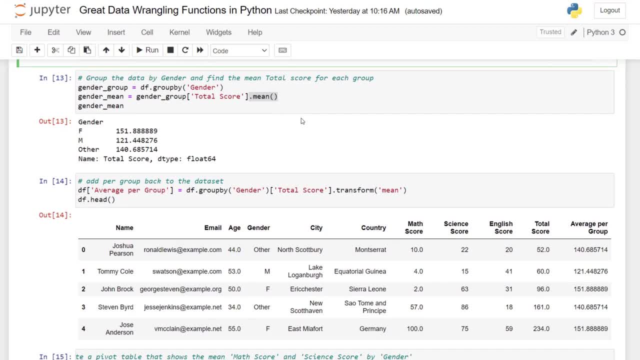 Next, what I want to do is create a group by, which is one of the most important data analyst functions out there, So you can group by your gender group. So I had a gender group by using DF. that group by You can also just add mean at the end of this and it will do the same thing as what I'm doing here, but I isolated the gender group. 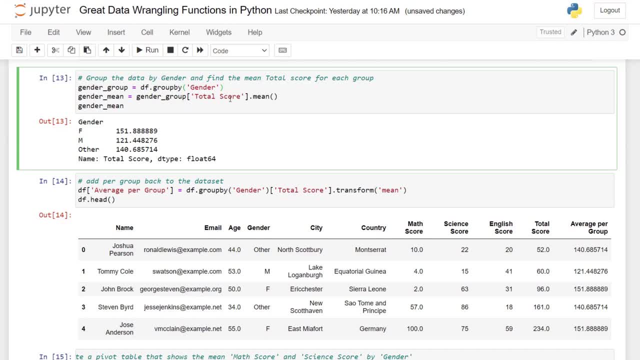 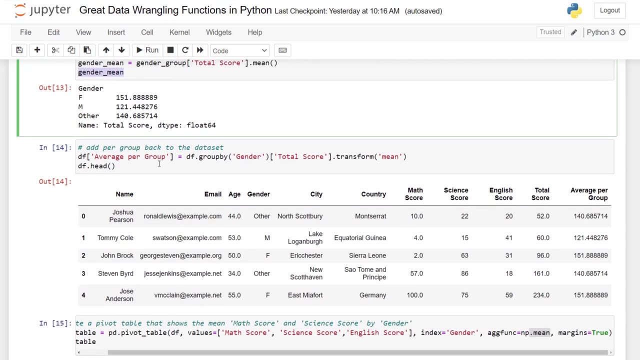 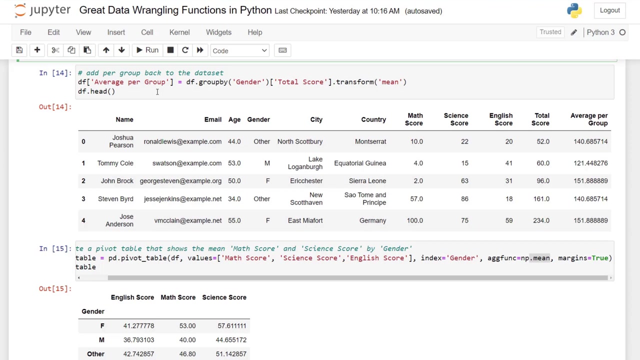 Then I added the total score Because I just want the total score mean, and then what we do is look at that, that variable, and what we have is the Mean of the genders- female, male and other. Next, I actually want to add the average per group back into our data set. 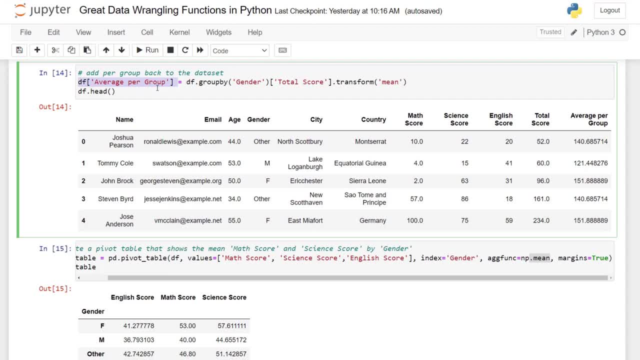 So I create a new column with the average per group and I use the group by isolate total score, I use the transform function and then I add mean. if we look at the head of the data set, you can see for each one of the particular genders: 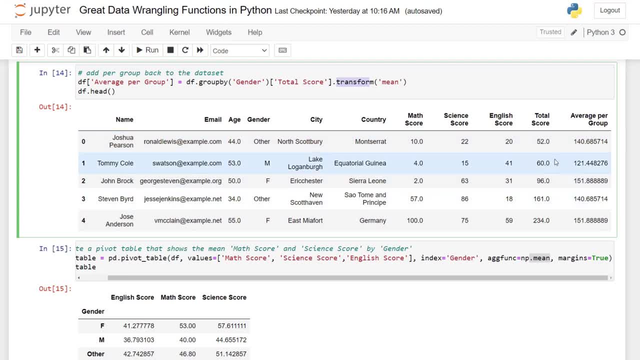 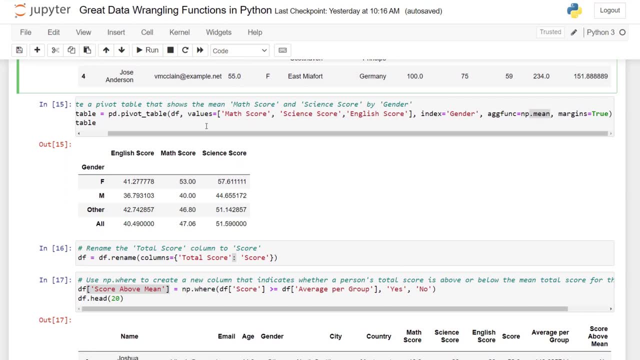 The average per that gender, and we want to do this so we can compare our total score to the average per group. But first you can create a pivot table. This is a very quick analysis that you can do. We use the pandas pivot table. 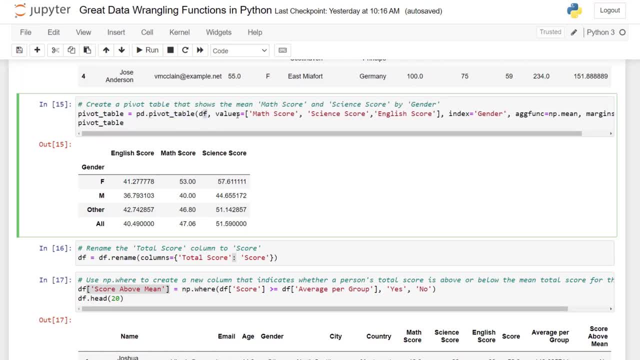 I just created a name called pivot table. We pass in our data frame, indicate the values that we want to aggregate our rows, or index is going to be gender And then I'm going to take the mean with MP dot mean You can change that to medium or some, or whatever you need. 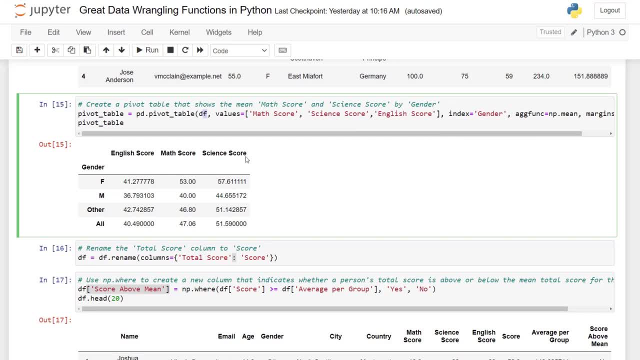 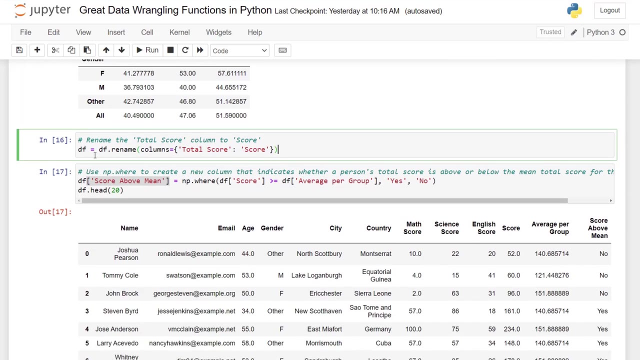 And I want the margins to be true so I can see the total. And this is what we end up with is a classic pivot table there, with all of the aggregated means. We can easily rename our total score column with score using a rename function. 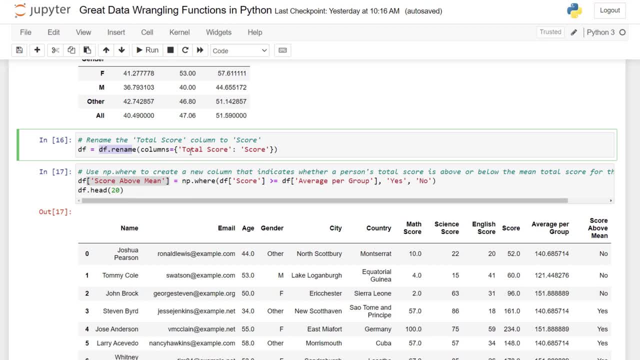 Pass in the columns with the bracket notation, And I use this with By indicating: I want the key of total score to be changed to the value score, And one of the last things we're going to do is compare our total score to the gender group mean. 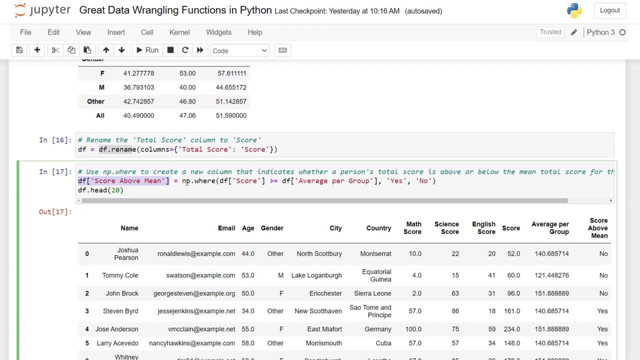 So I'm going to create a new column called score, above mean. I'm going to use that numpy function where, which is a conditional. This is going to allow me to create a comparison. So anything that we have A score greater or equal to the average per group. 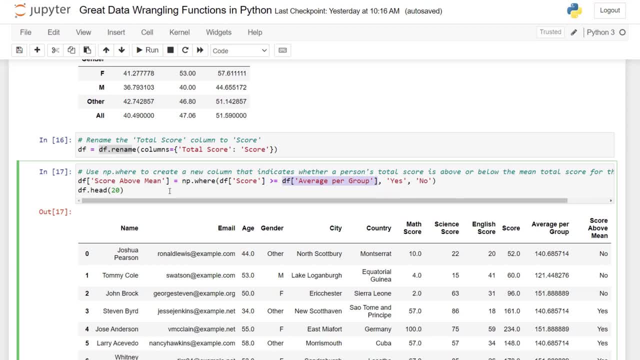 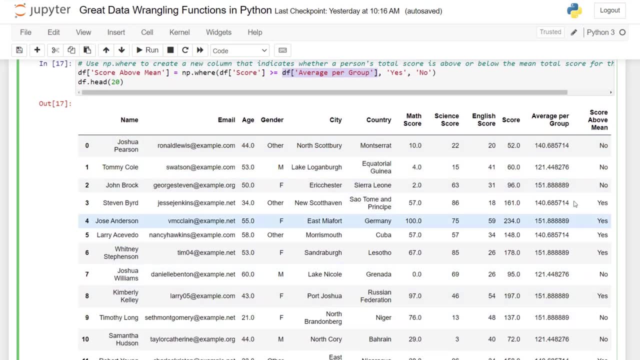 Give me a yes or no if it's lower, And then let me look at the first 20 that are there And, as you can see, we get the average per group column here that we created previously. We have our score and then we do the evaluation: whether it's higher or lower.